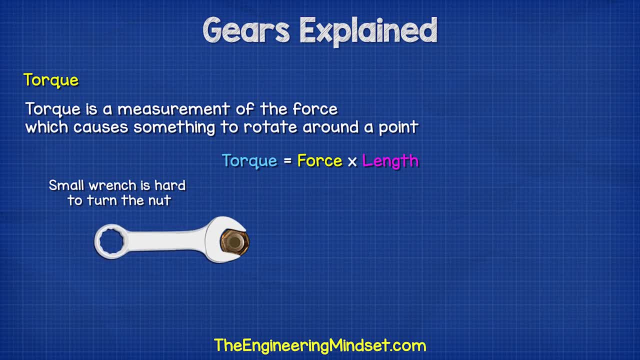 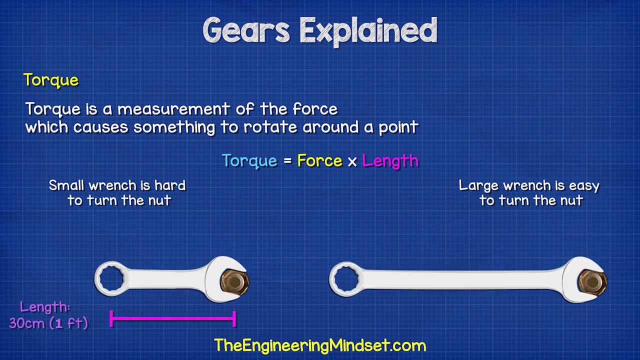 Using a small wrench is very hard. Using a long wrench will make it much easier. That's because of torque. If we used a 30cm wrench and applied 90N of force, we have 0.3m multiplied by 90N, which gives us 27Nm of torque. 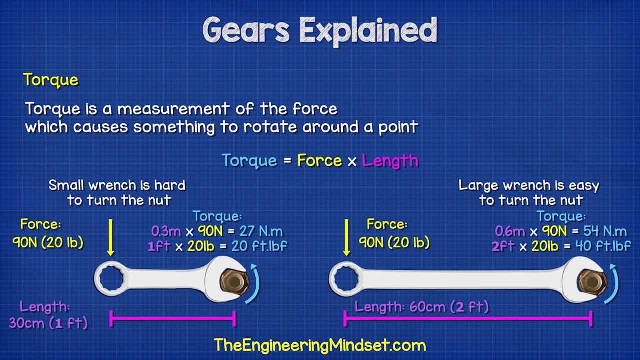 However, if we applied the same 90N of force to a wrench that was 60cm long, then we would get 0.6m. If we applied the same 90N of force to a wrench that was 60cm long, 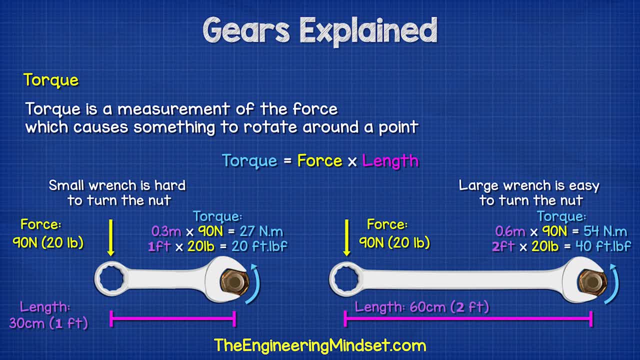 then we would get 0.3m multiplied by 90N, which gives us 54Nm. So from this simple formula you can see we have more force acting on the nut by using a longer wrench. Essentially, we're using a larger circle to turn a smaller circle. 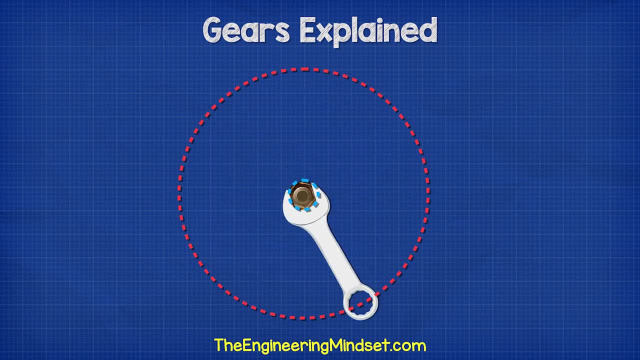 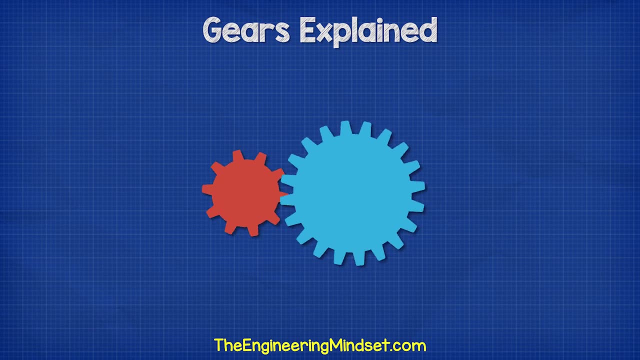 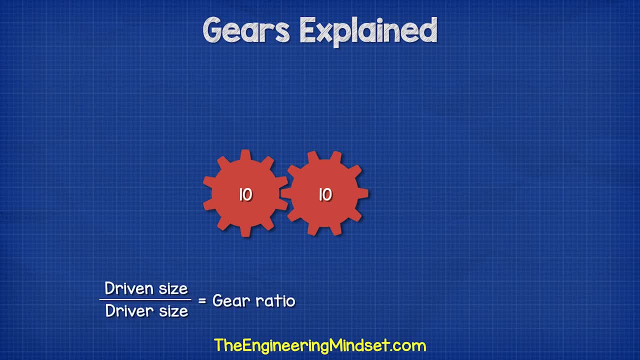 If we attach the other gear to the other gear, then the other gear would also rotate. If we attach the other gear to the other gear, then the other gear would also rotate. we have a one-to-one ratio, which means every time the driver gear 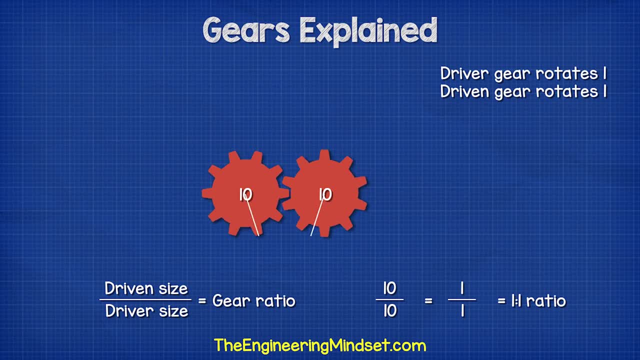 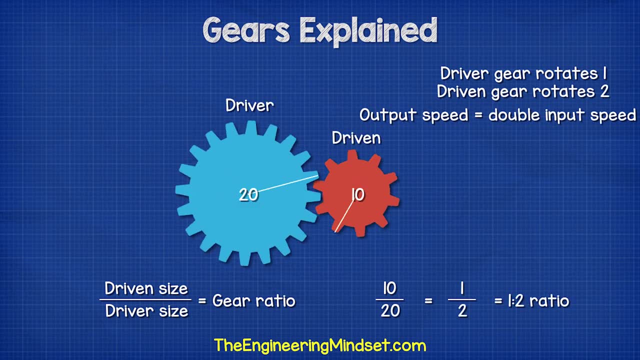 completes a full rotation, the driven gear also completes one rotation, So the output speed is the same as the input speed. If the driven gear is half the diameter of the driver gear, then we have a one-to-two ratio, which means for every full rotation of the driver gear. 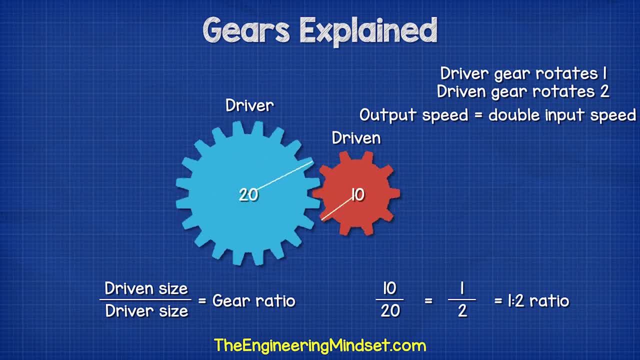 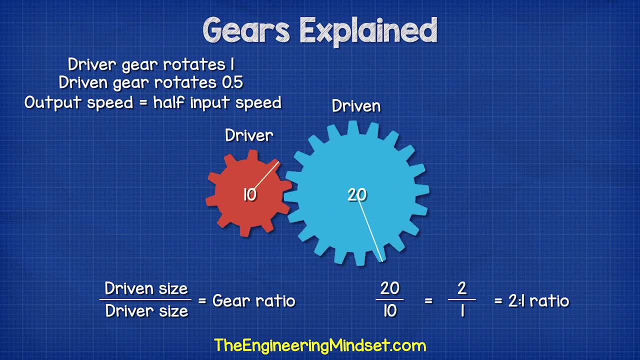 the driven gear completes two full rotations. This means the driven gear is rotating much faster. If the driven gear is twice the diameter of the driver gear, then we have a two-to-one ratio, which means for every one full rotation of the driver gear. 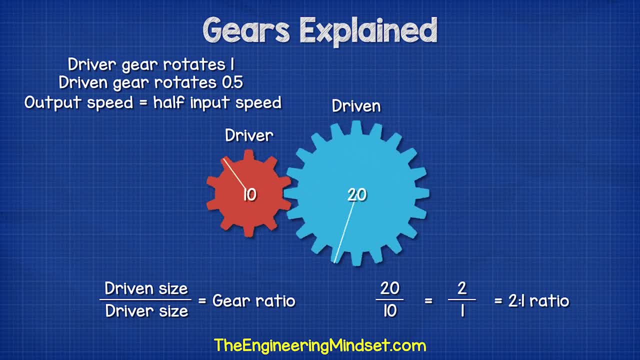 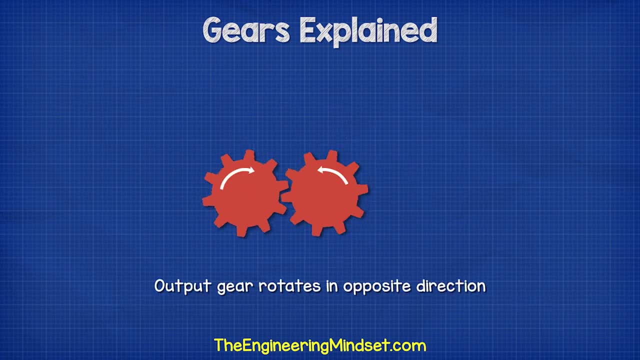 the driven gear rotates only half a turn, So we need the driver gear to rotate twice to complete a full rotation of the driven gear. Notice that the driven gear rotates the opposite way. This is basically a reverse gear In order to make the output rotate. 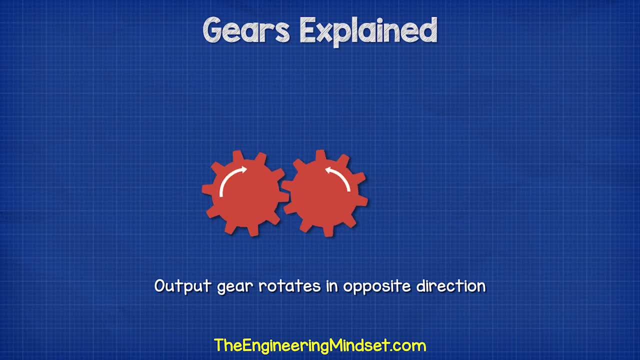 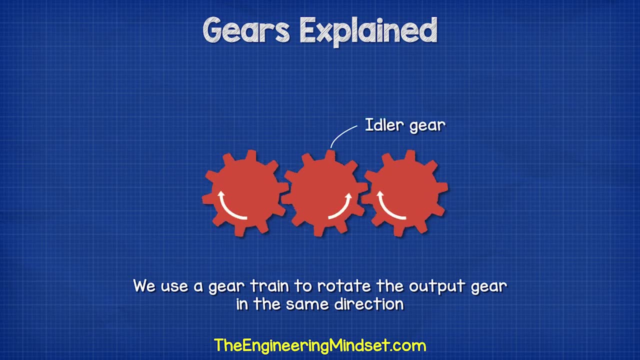 in the same direction as the input, we need to insert another gear which creates something known as a gear train. The middle gear is known as an idler gear. We could add many gears side by side to change the speed and also the output direction. 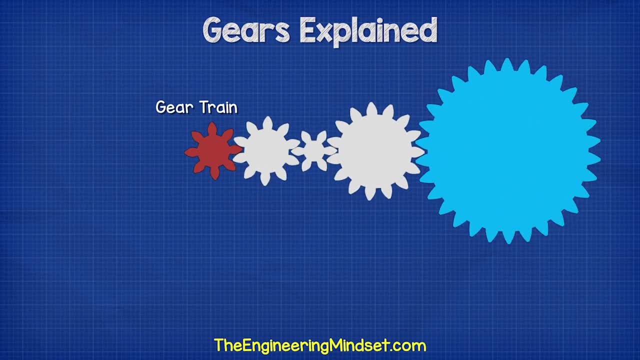 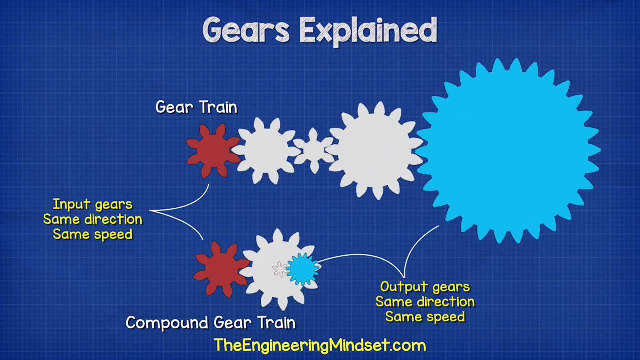 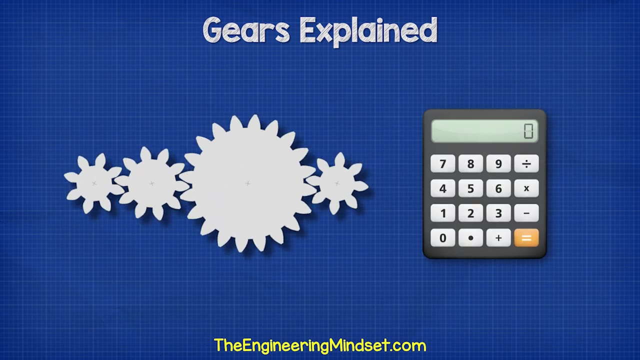 but this will take up a lot of room. So instead we can mount gears to the same axis and create a compound gear train. This will do the same job, but it will take up far less space. Let's look at how to calculate the RPM and torque. 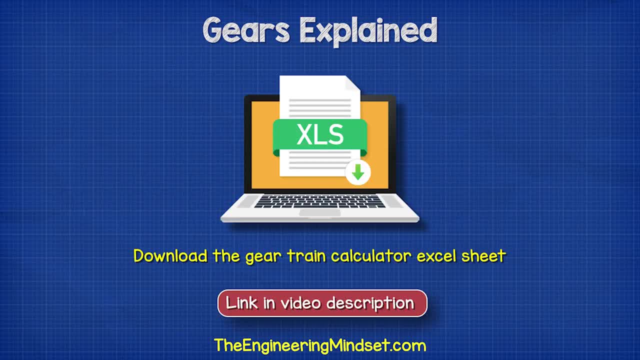 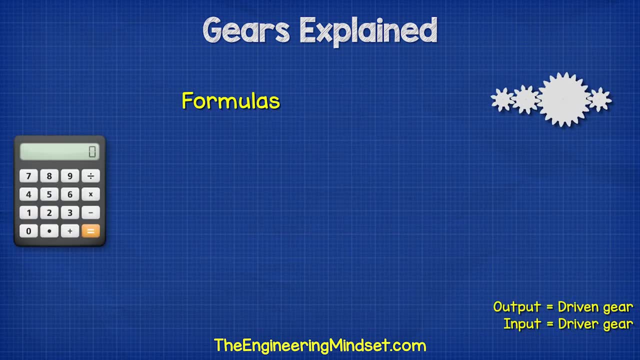 of simple gear trains. By the way, you can download an Excel sheet of these calculations. Links can be found in the video description. for those We're going to use the formulas. ratio equals teeth of the output gear divided by teeth of the input gear. 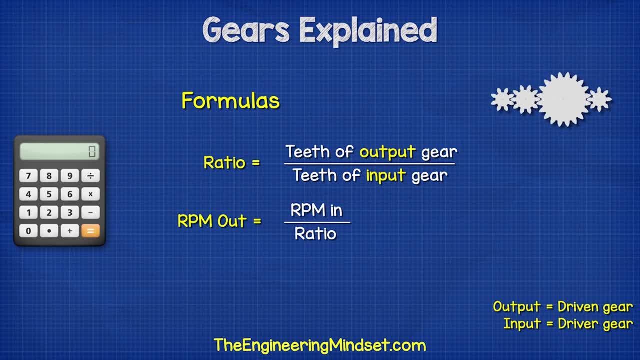 RPM output equals the output gear. RPM output equals the output gear. RPM input divided by the ratio. And finally, torque output equals the ratio multiplied by the torque input. For example, if gear A has 8 teeth and gear B has 10 teeth, 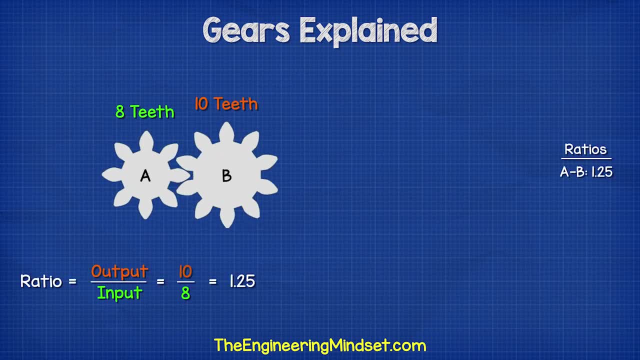 the ratio is 10 divided by 8, which is 1.25.. If gear A rotates at 150 RPM, then 150 divided by 1.25 equals 120.. If gear A has a torque of 20 Nm, 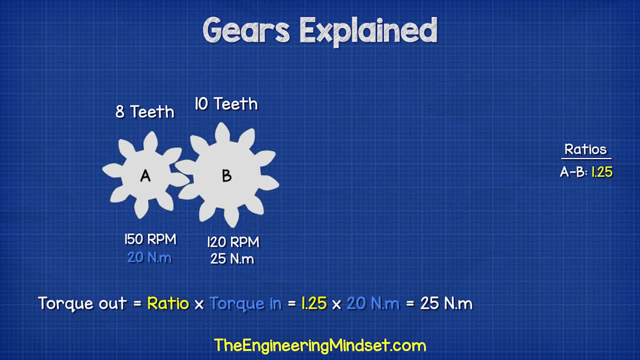 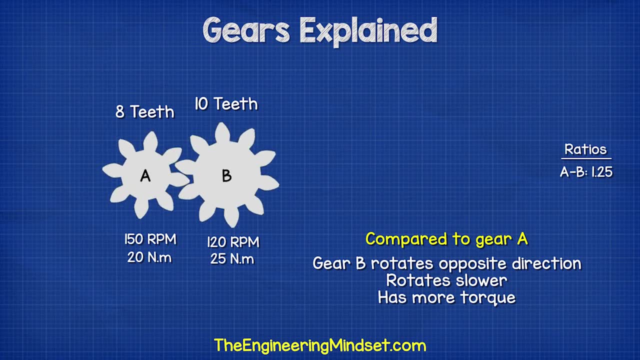 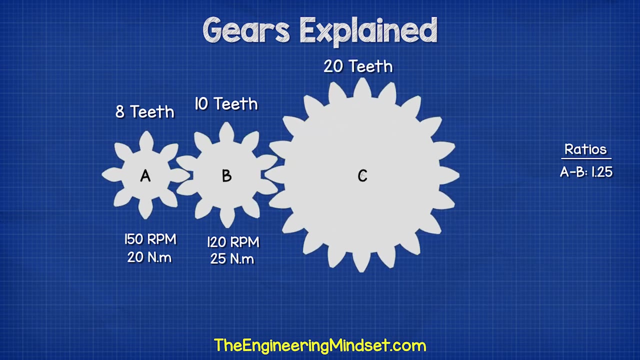 then 1.25 multiplied by 20 gives us 25 Nm. This gear will rotate the opposite way to gear A. It will rotate slower because it is larger, but it will have more torque. If we add gear C with 20 teeth, 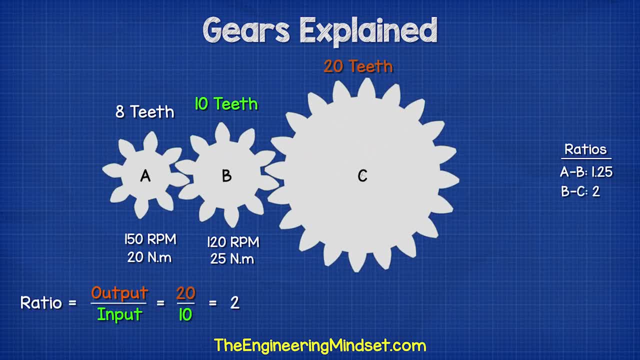 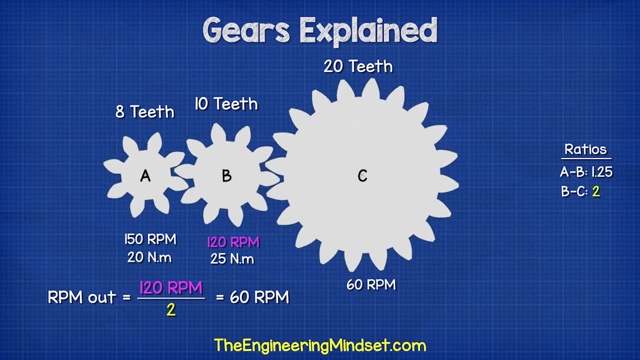 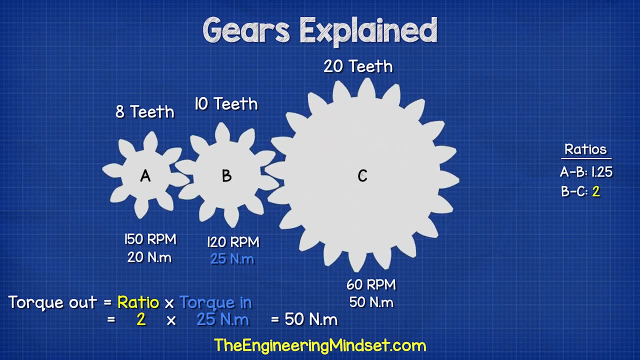 the ratio is 20 divided by 10, which gives us 2.. The RPM output is 120 RPM. from gear B divided by 2, which gives us 60 RPM. The torque is going to be 2 multiplied by 25 Nm. from gear B. 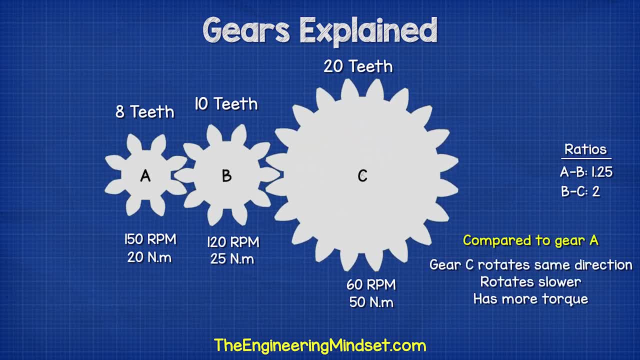 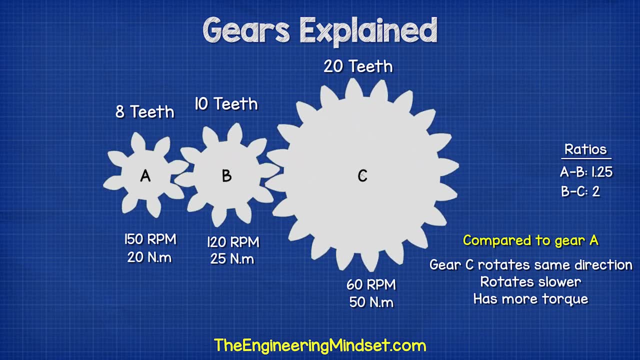 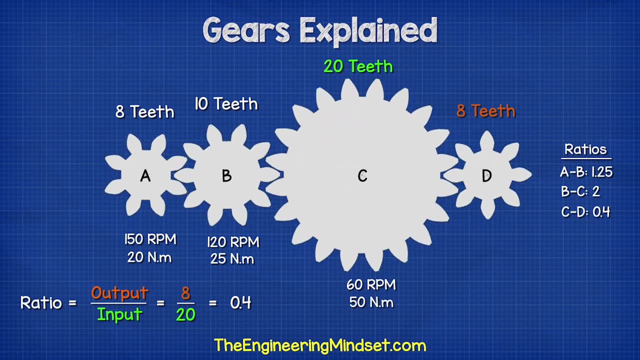 This will give us 50 Nm. So this gear will rotate the same direction as gear A, but it will rotate slower because it is larger, although it will have more torque. If we were to add gear D with 8 teeth, then the ratio is 8 divided by 20,. 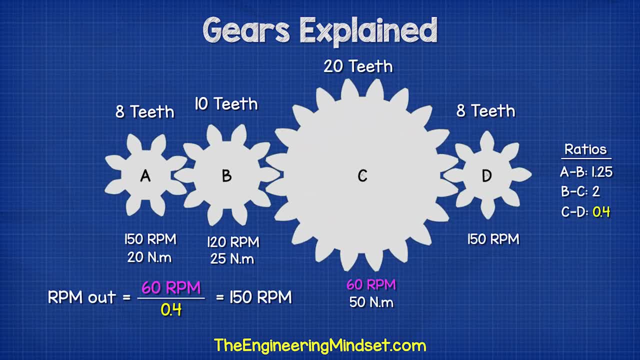 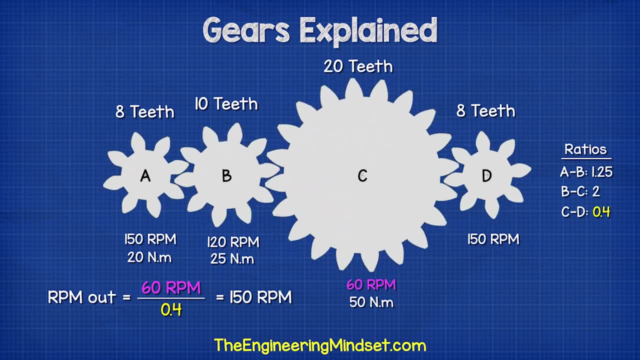 which gives us 0.4.. The RPM is 60 RPM from gear C divided by the ratio of 0.4,, which gives us 150 RPM. The torque is 0.4 multiplied by 50 Nm, which gives us 20 Nm. 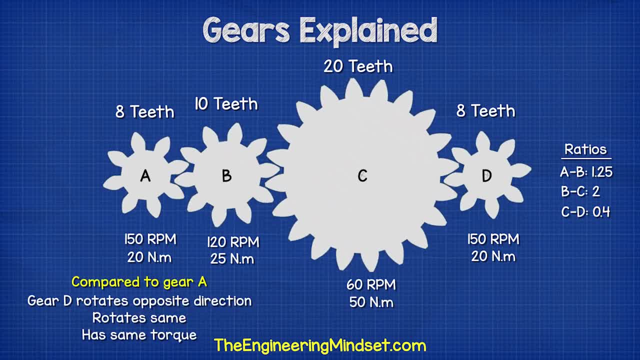 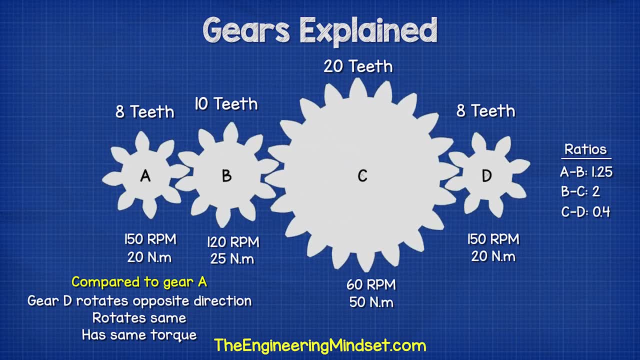 So this gear will rotate the opposite way to gear A, but it is the same size, so it will rotate at the same speed and the same torque, although this doesn't take into account any losses which we would see in the real world. So this setup lets you visualize. 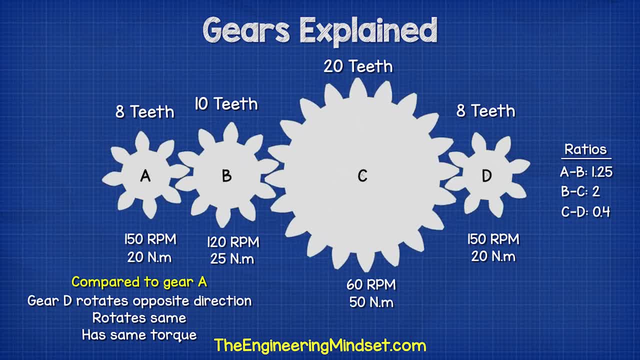 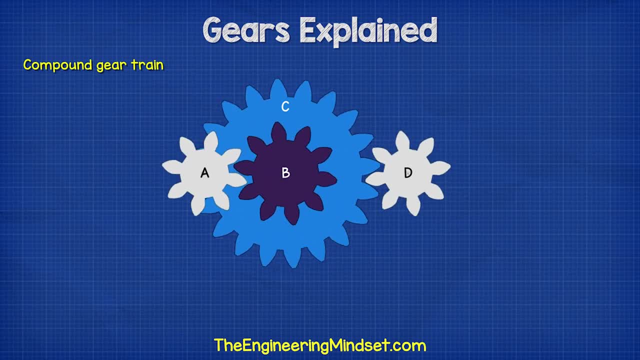 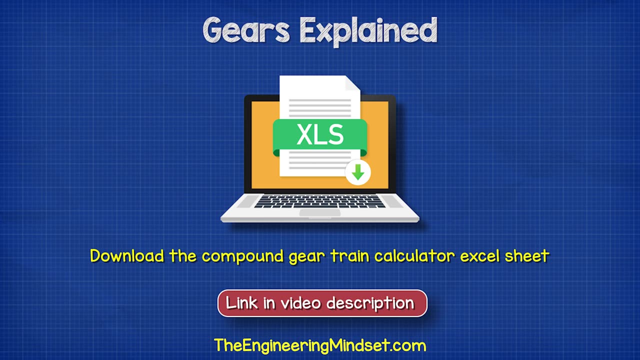 how gears manipulate speed, torque and direction. What if we had a compound gear train like this which has the same size gears, the same input torque and the same rotational speed? Again, links in the video description for the Excel sheet calculator for this: 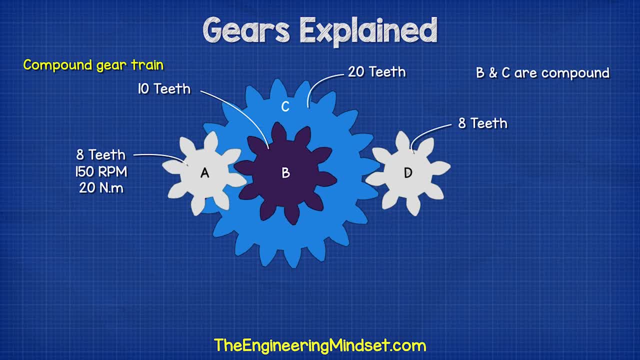 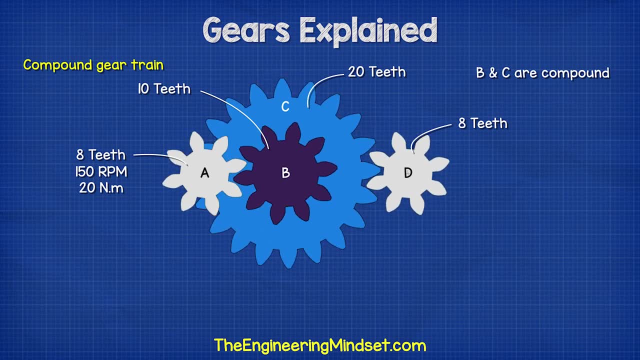 So with this setup we have 4 gears: A, B, C and D. but B and C are compound. If gear A has 8 teeth and gear B has 10 teeth, then the ratio is 10 divided by 8,. 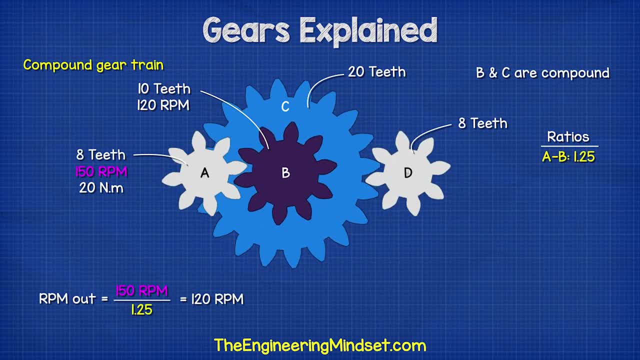 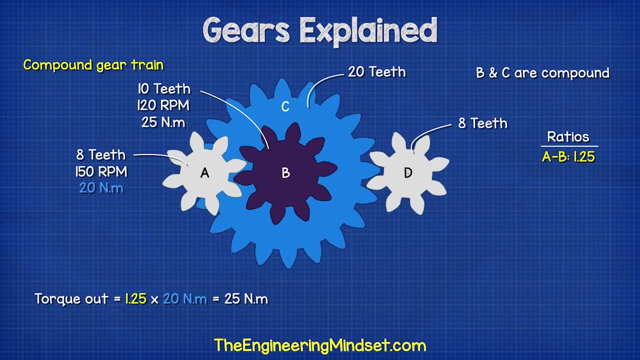 which is 1.25.. Gear A rotates at 150 RPM, so gear B is 150 RPM divided by 1.25, which gives us 120 RPM. Gear B has a torque of 20 Nm, so gear B is 1.25 multiplied by 20 Nm. 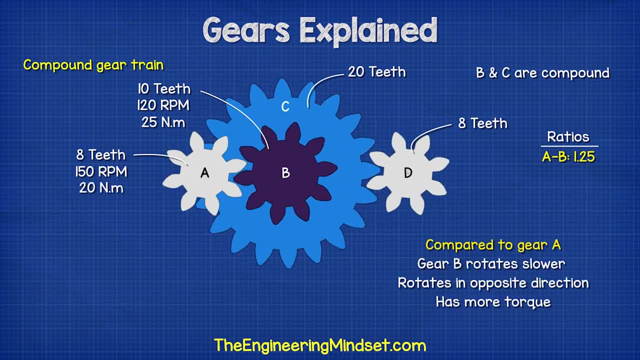 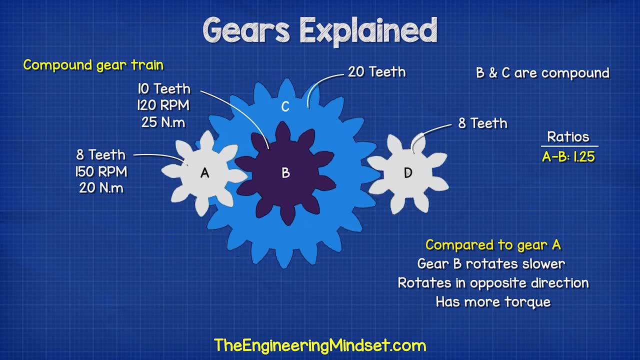 which is 25 Nm. So this gear rotates the opposite way to gear A. it will rotate slower because it is larger, but it has more torque. If gear C has 20 teeth, then the ratio is 20 divided by 10,. 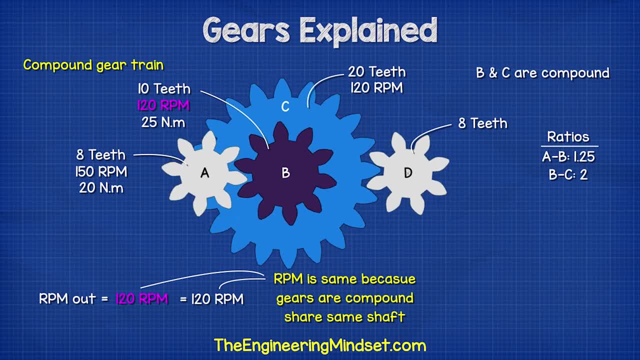 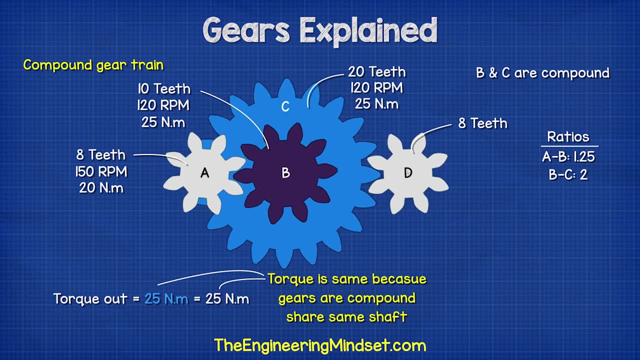 which is 2.. The RPM is going to be the same as B, which is 120 RPM, because these two gears are compound and share the same shaft. The torque is also going to be the same as B, so it's 25 Nm.